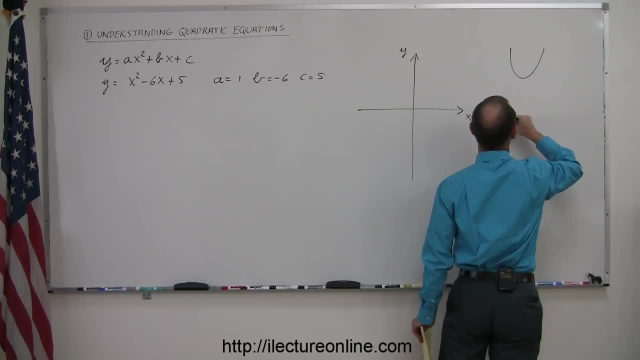 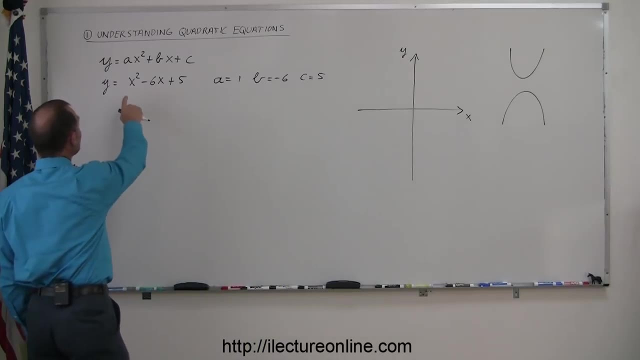 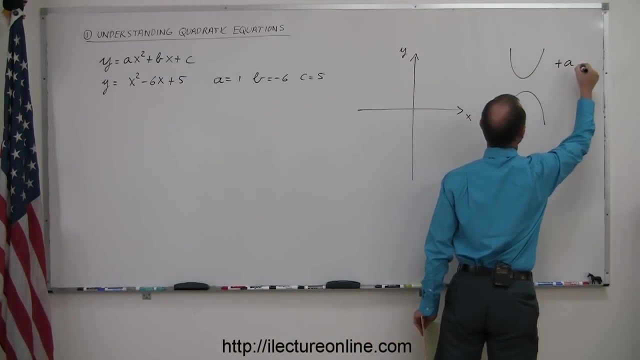 will be graphed. either it will look like this or it will look like that, And the way you can tell if it's going to open upward or open downwards we call it- is: if the number in front of the x squared term is positive, it'll look like this: So that's a plus a, and if the number in front of the x squared term is negative, it'll look like this: So that's a plus a. and if the number in front of the x squared term is negative, it'll look like this: So that's a plus a. and if the number in 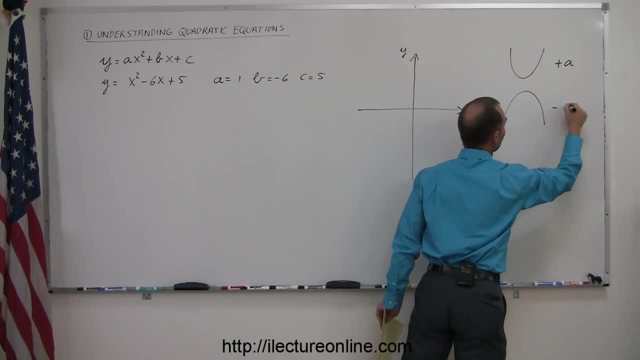 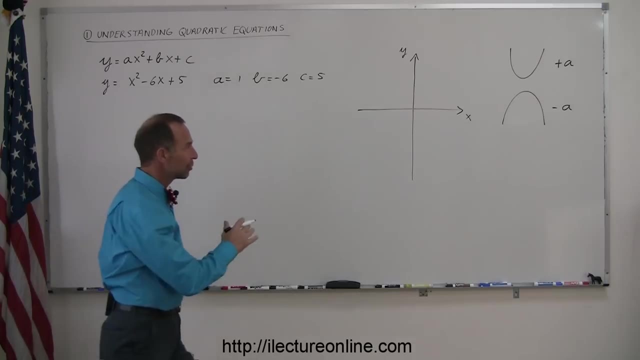 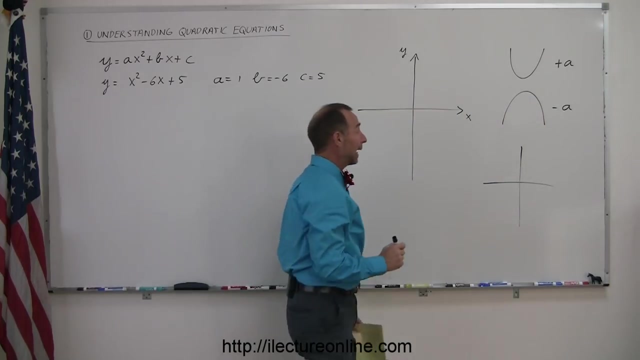 negative, then it'll look like this. so think of it as a minus a. All right, that helps us a little bit. Now also realize that if you graph these, that this parabola, as we call them, these graphs for quadratic equations called parabolas, and it could potentially 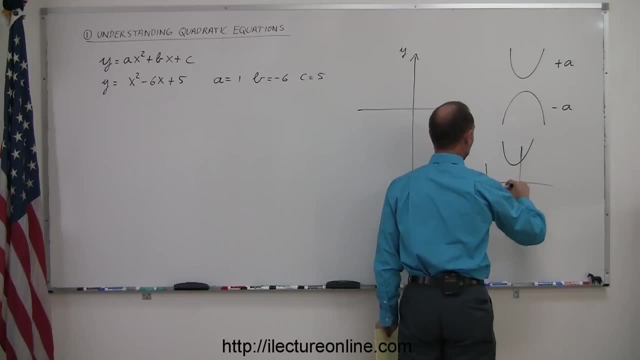 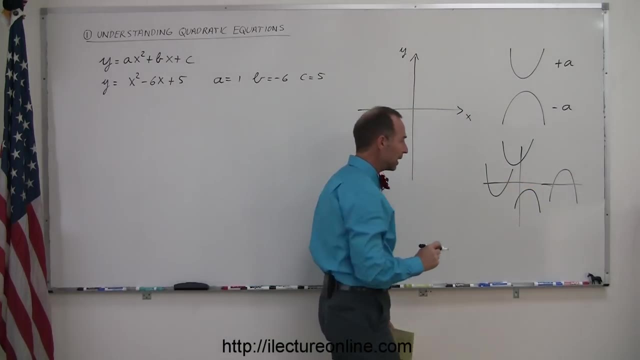 if we were to graph it, it could end up looking like this, or it could end up looking like this, or it could end up looking like that, or maybe it looks like this, And notice that in some cases, the parabola will cross the x-axis, like this particular parabola will. 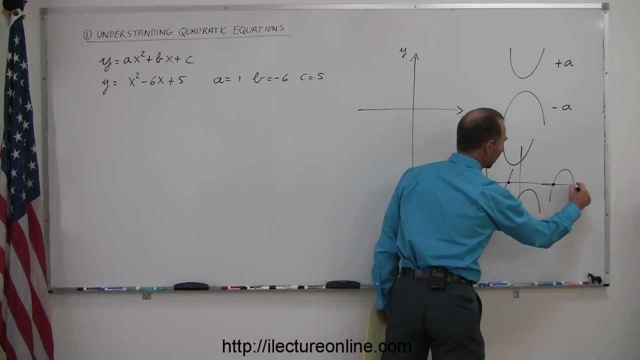 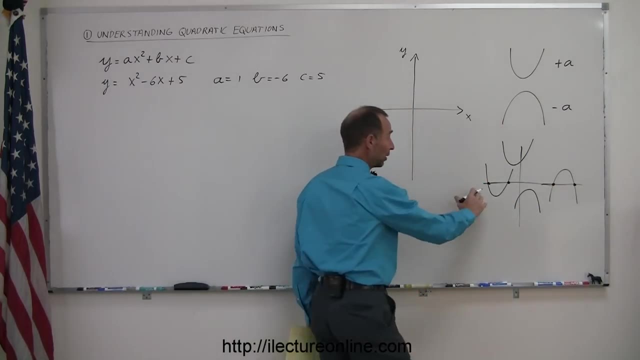 cross it in two places. this particular parabola will cross it in two places, and these two parabolas do not cross the x-axis at all: The places where one of these parabolas, which is a graphical representation of a quadratic equation like this, where the parabola crosses. 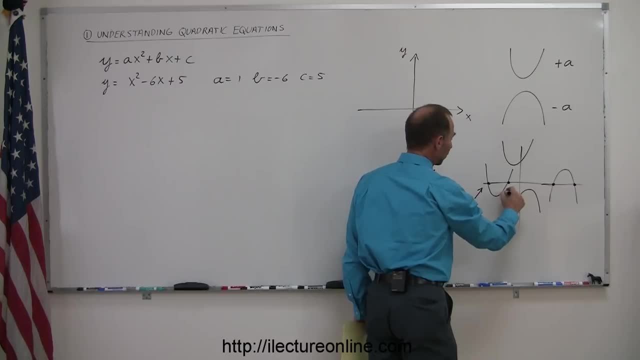 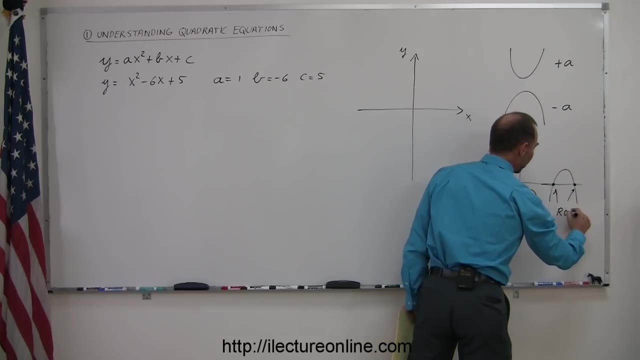 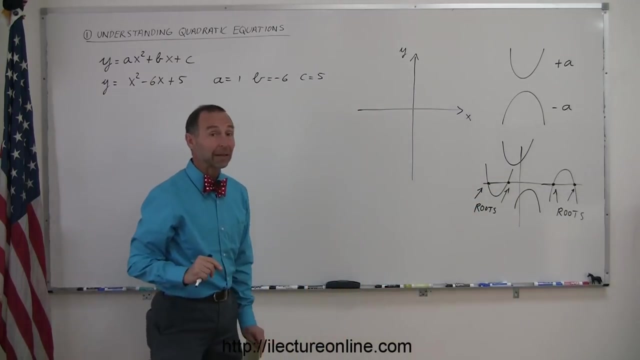 the x-axis. those are called the roots of the quadratic equation. So we call these roots, And here again these would be considered the roots of the quadratic equation. Notice that these two do not have roots. So sometimes when they ask you to solve, 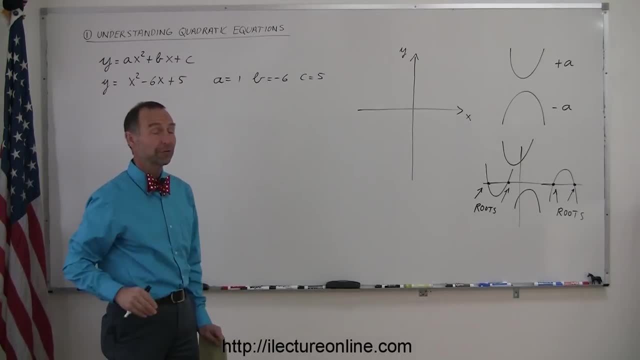 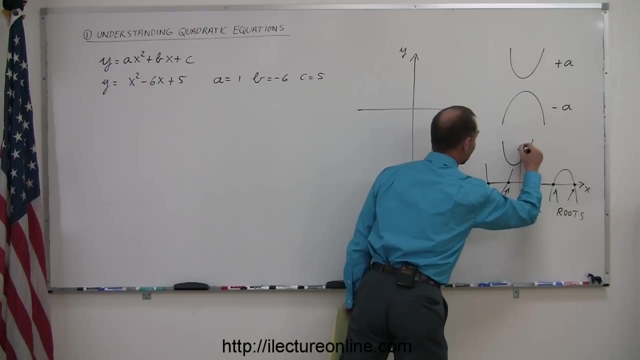 a quadratic equation. they're basically asking you to find the roots of the parabola and, of course, if the parabola does not cross the x-axis- like again, this is here the x-axis, this here is the y-axis, like in this case, or in this case- then there's no solution. 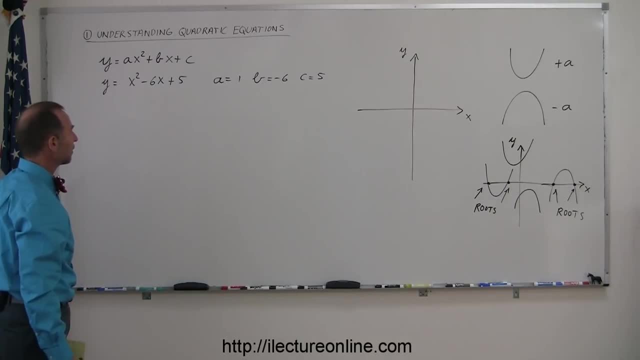 there are no roots. So the problem is that the parabola is not a quadratic equation. So to help us figure out what it actually is and how to graph these quadratic equations, let's go ahead and factor this. This happens to be a factorable equation, so we can write. 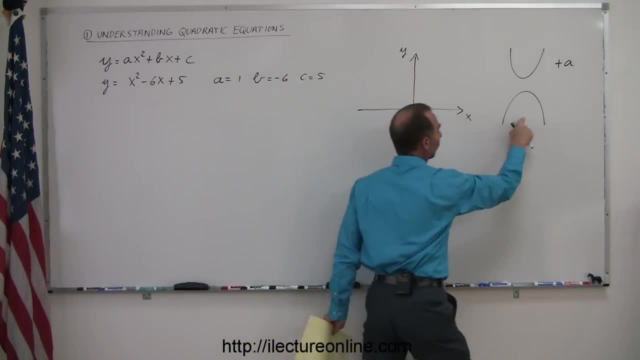 the x squared term is negative, it'll look like this: So that's a plus a, and if the number in negative, then it'll look like this. so think of it as a minus a. All right, that helps us a little. 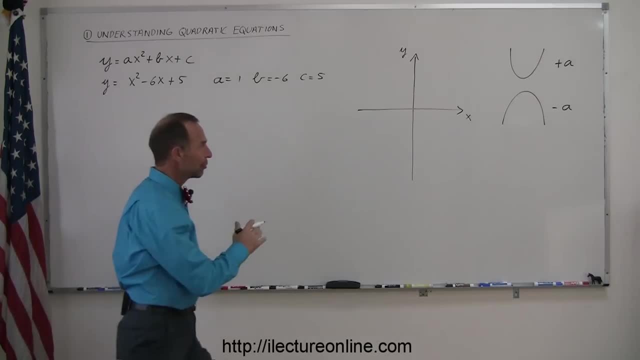 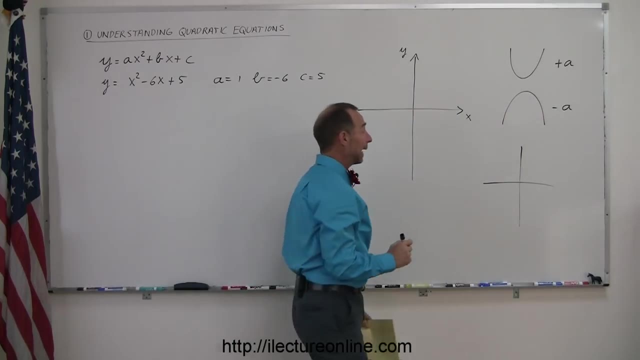 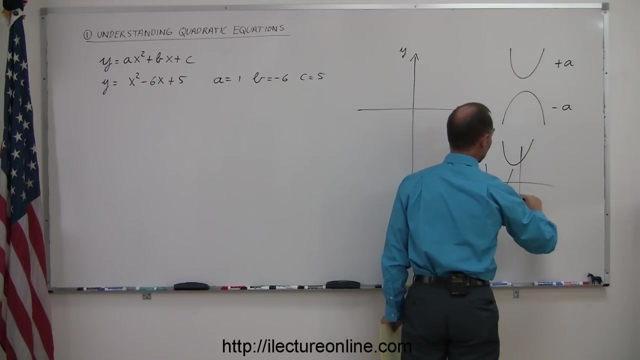 bit. Now also realize that if you graph these, that this parabola, as we call them, these graphs for quadratic equations called parabolas, and it could potentially, if we were to graph it, it could end up looking like this, or it can end up looking like this, or it can end up looking like that. 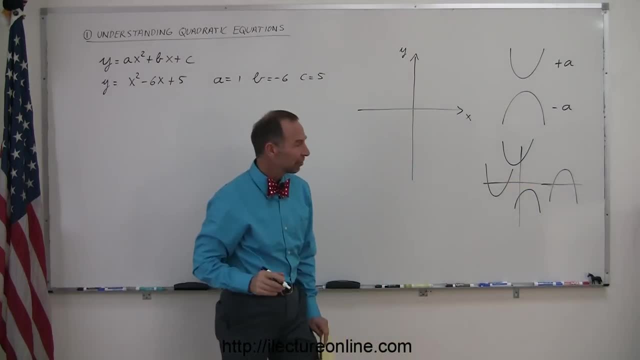 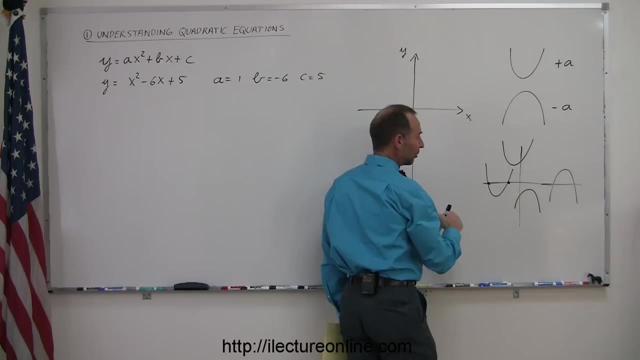 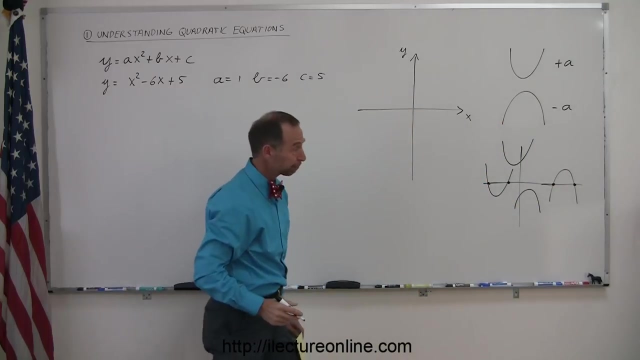 or maybe it looks like this, and notice that in some cases the parabola will cross the x-axis, like this particular parabola will cross it in two places. this particular parabola will cross it in two places and these two parabolas do not cross the x-axis at all The places where 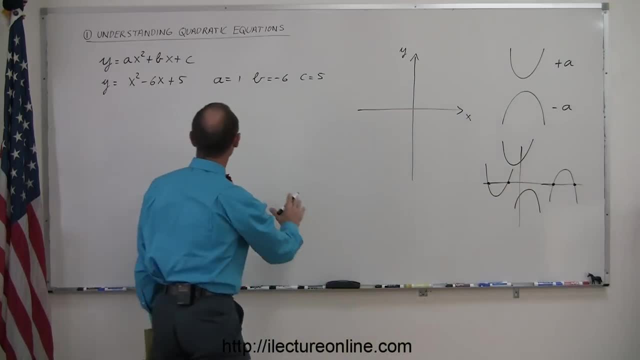 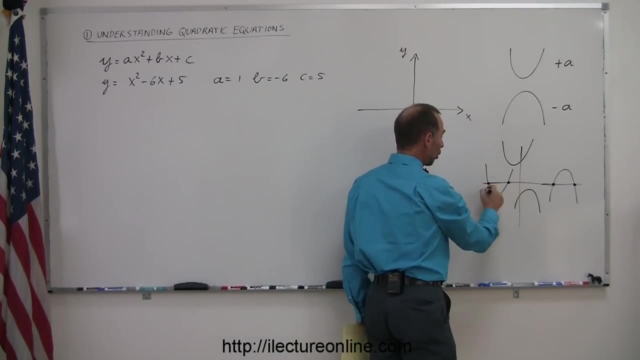 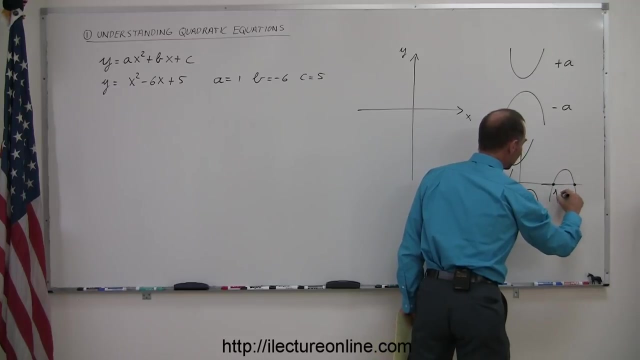 one of these parabolas, which is a graphical representation of a quadratic equation like this, where the parabola crosses the x-axis, those are called the roots of the quadratic equation. so we call these roots, and here again these would be considered the roots of the quadratic equation. Notice that these two 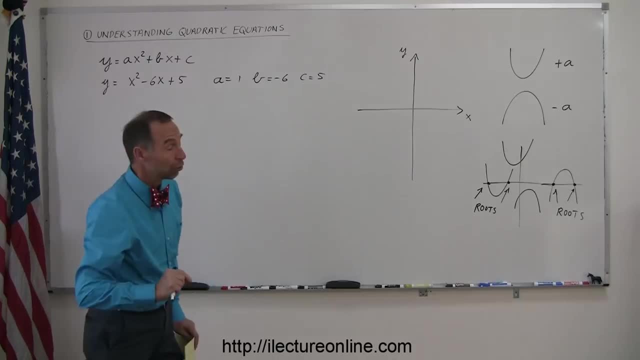 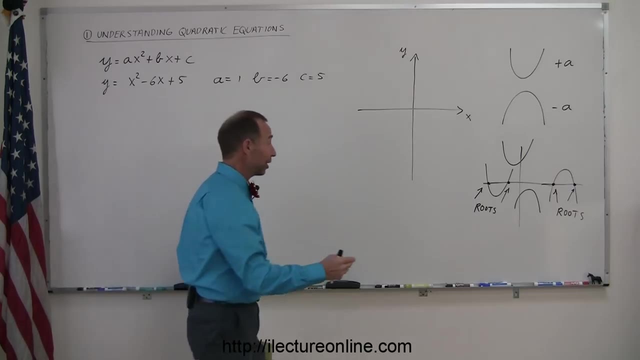 do not have roots. so sometimes, when they ask you to solve a quadratic equation, they're basically asking you to find the roots of the parabola and, of course, if the parabola does not cross the x-axis, like again, this is here the x-axis, this here is the y-axis. 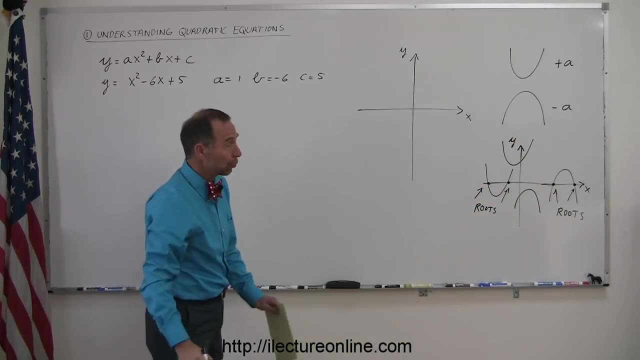 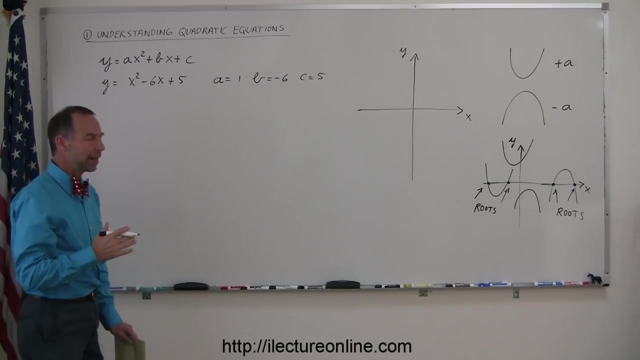 like in this case. in this case, then, there's no solution, there are no roots to the quadratic equation. All right, so to help us figure out what it actually is and how to graph these quadratic equations, let's go ahead and factor this. this happens to be a factorable equation, so we can write this as: y is equal to. 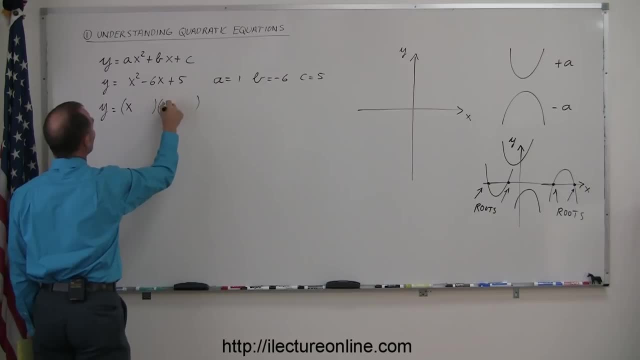 the product of two binomials. we write the x and the x, since there's a negative here and a positive there. that means one must be plus and one must be negative or no. in that case, I'm sorry. actually they both must be negative. 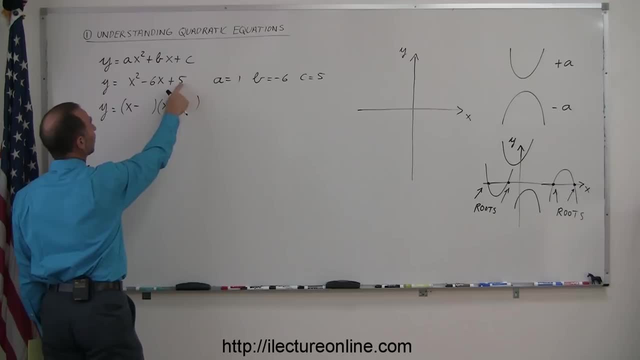 negative, because the only way you can get a positive number there is either that you have two positive numbers here or two negative numbers, and since this is negative, you have to have two negative numbers. so now we're looking for two numbers. when you multiply them, you get a five. 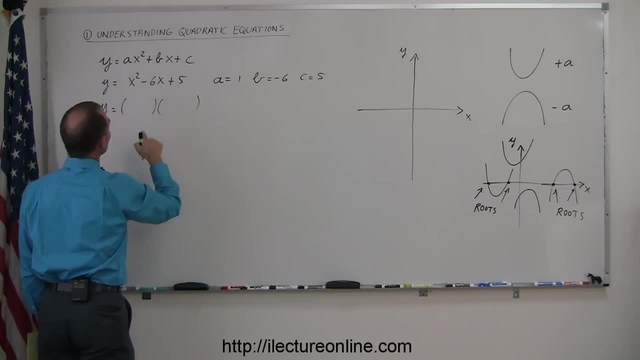 this: as y is equal to the product of two binomials, we write the x and the x, since there's a negative here and a positive there. that means one must be plus and one must be negative or no. in that case, I'm sorry. 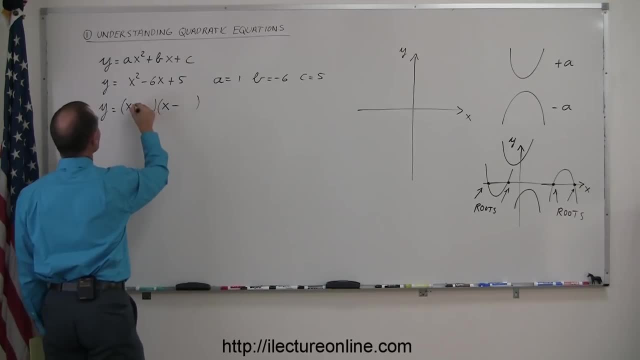 Actually they both must be negative, because the only way you can get a positive number there is either that you have two positive numbers here or two negative numbers, and since this is negative, you have to have two negative numbers. So now we're looking for. 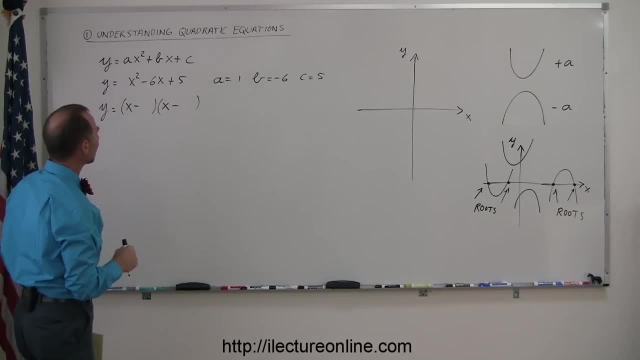 two numbers. when you multiply them, you get a five. when you add them, you get a six. so it looks like a five and a one, because if I multiply x times a negative one and multiply negative five times an x and add them together, I get negative six, x my middle term. All right, 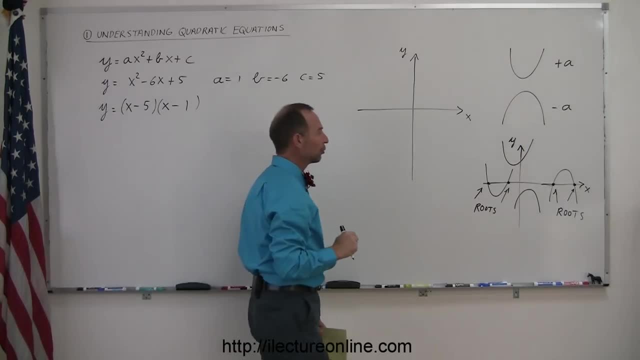 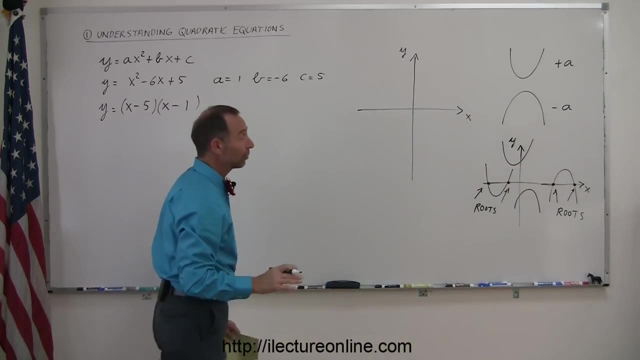 Now, if we want to solve a quadratic equation or find the roots, realize that the roots are the points that lie on the x-axis. that means that at that location the y value is equal to zero. So any point on the x-axis my y value is zero, which means that if I'm 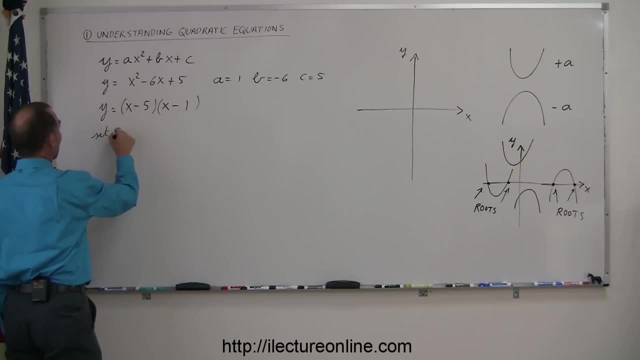 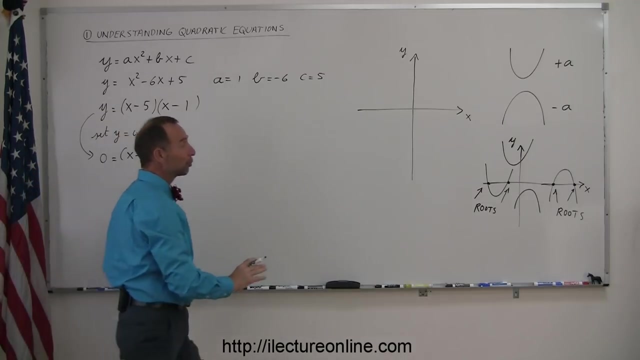 going to find the roots. I'm going to set my y equal to zero. If I do that, this equation now becomes zero is equal to x minus five times x minus one, And if I solve the quadratic equation, I solve this for x. then I will find the points where the equation crosses. 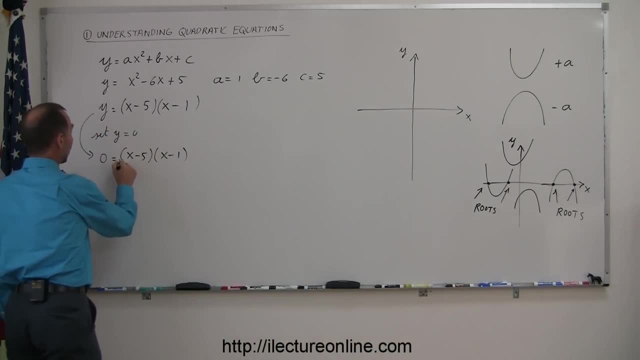 the x-axis. All right Now, if I have two quantities multiplied together and the solution is zero, that means either one or the other must be zero, because the only way you can multiply two things together and get zero is if either x minus five equals zero or the x minus one. 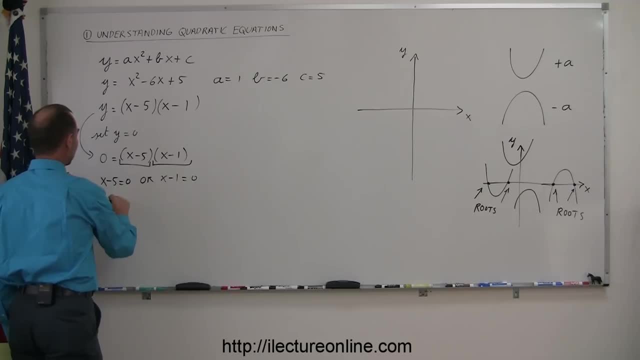 equals zero. And, of course, if x equals x minus five equals zero, then x must equal five. or if x minus one equals zero, then x must equal one. And those are the locations in this particular example where the parabola will cross the x-axis. 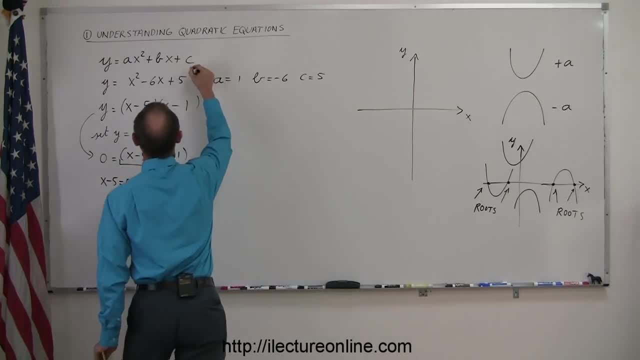 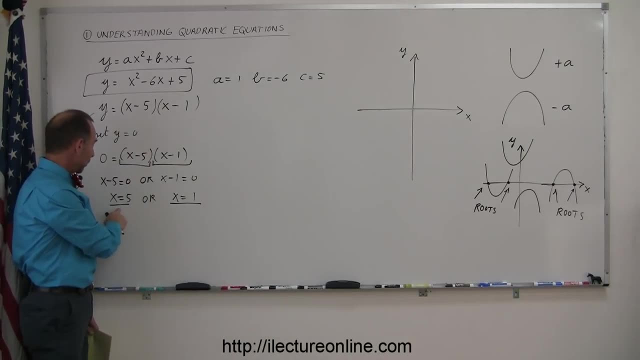 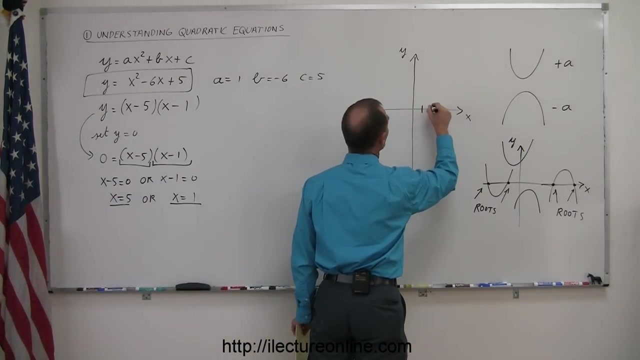 So if I'm going to graph what I have here, my example, if I'm going to graph this example on my x-y-axis here, I know that one of the roots or one of the points where the graph will cross the x-axis, x equals five, one, two, three, four, five, six, seven, eight. 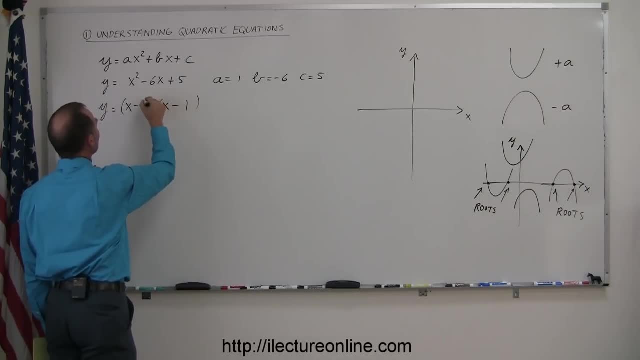 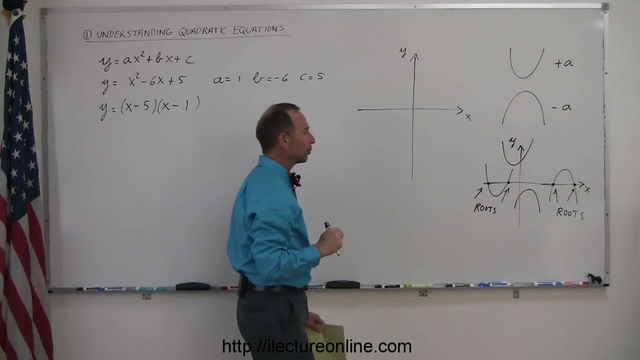 when you add them you get a six, so it looks like a five and a one, because if I multiply x times a negative one and multiply a negative five times an x and add them together, I get negative six, x, my middle term. all right now, if we want to solve a quadratic equation or find the roots. 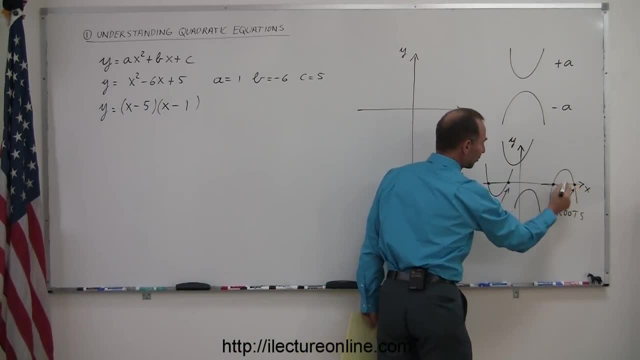 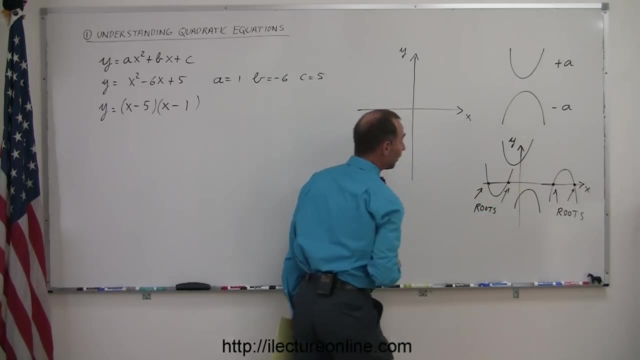 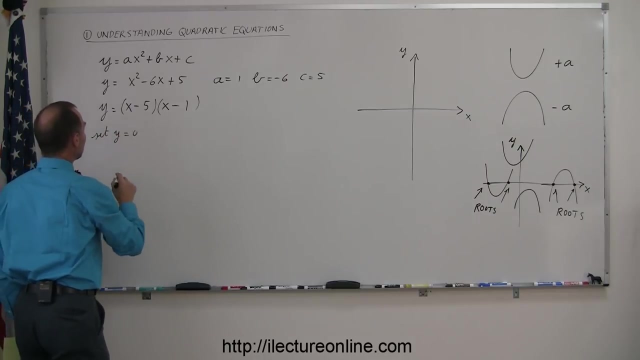 realize that the roots are the points that lie on the x-axis. that means at that location the y value is equal to zero. so any point on the x-axis my y value is zero. which means if I'm going to find the roots, I'm going to set my y equal to zero. if I do that, this equation now. 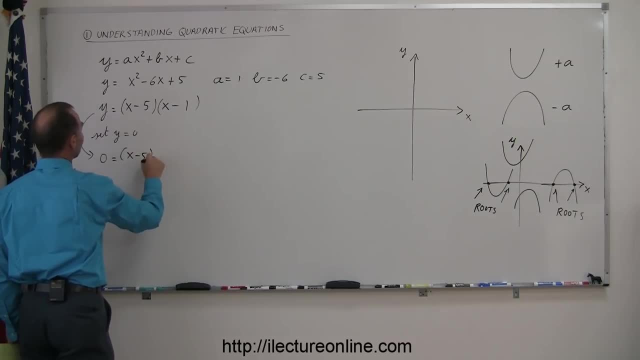 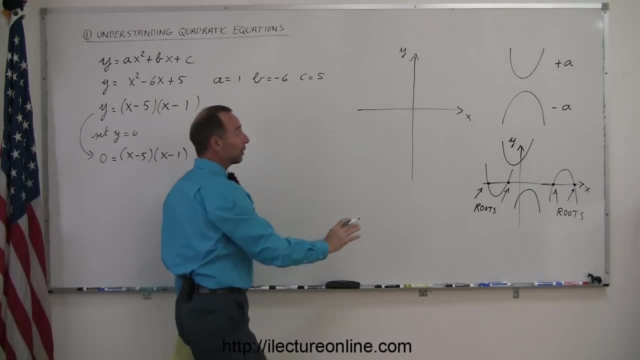 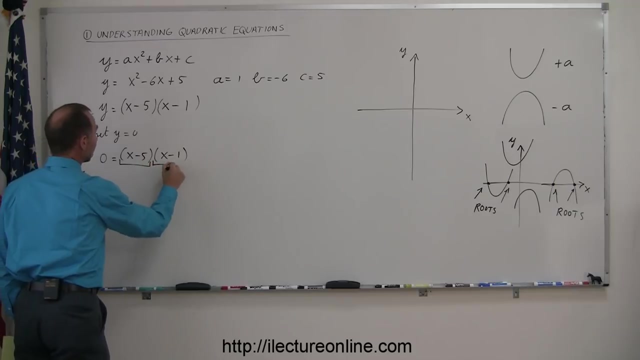 becomes zero is equal to x minus five times x minus one, and if I solve this for x, then I will find the points where the equation crosses the x-axis. all right now, if I have two quantities multiplied together and the solution 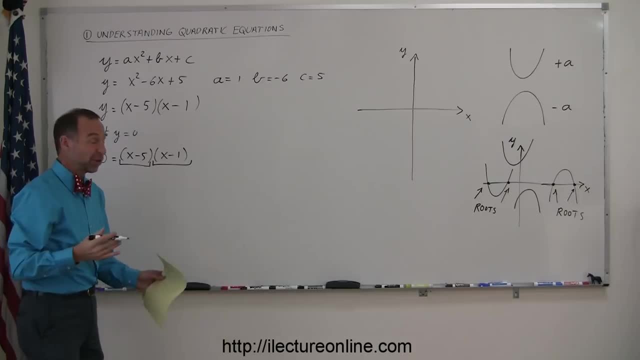 is zero. that means either one or the other must be zero, because the only way you can multiply two things together and get zero is if either x minus five equals zero or the x minus one equals zero, and, of course, if x equals x minus five. 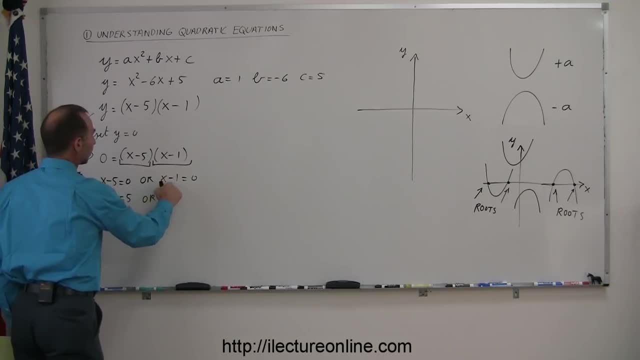 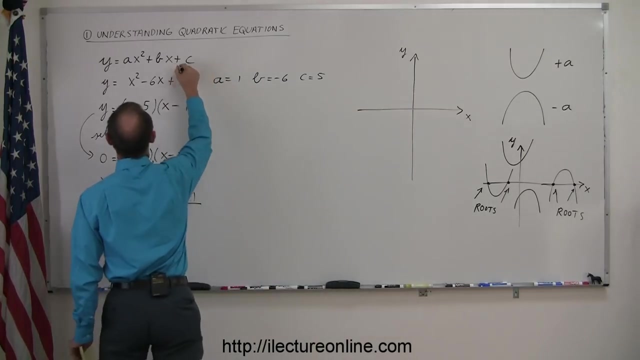 then x must equal five. or if x minus one equals zero, then x must equal one. and those are the locations in this particular example where the parabola will cross the x-axis. so if I'm going to graph what I have here, my example, if I'm going to graph this example on my xy-axis, here I know. 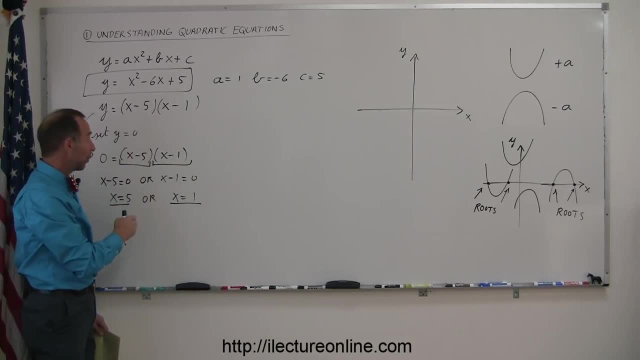 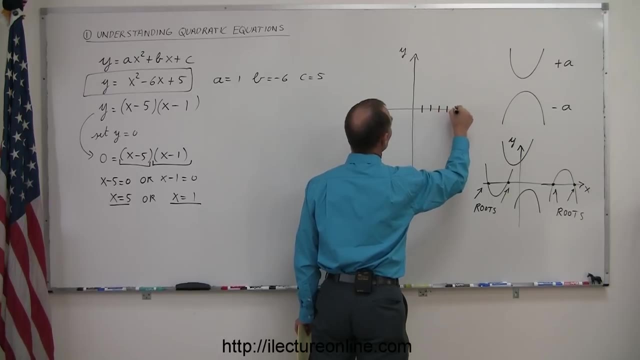 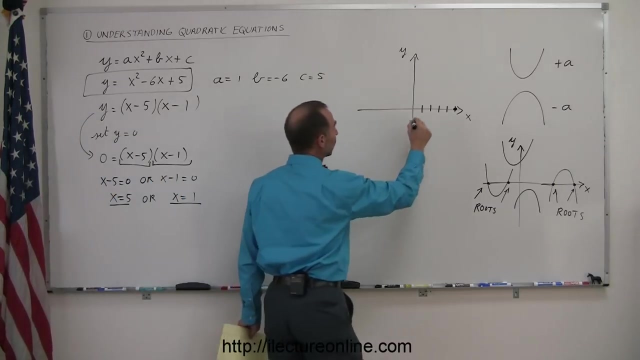 that one of the roots or one of the points where the graph will cross the x-axis, x equals five, one, two, three, four, five, so right there. and the other place where it crosses the x-axis will be at x equals one, which is right here, and those are considered the two roots of my quadratic equation. 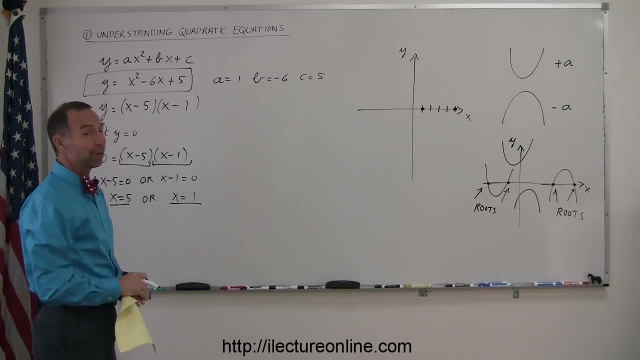 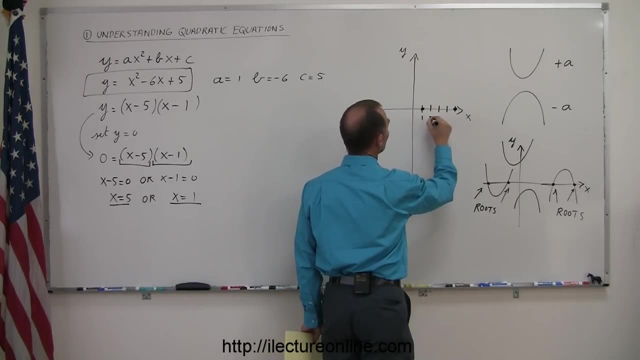 All right. now there's another thing about a quadratic equation that's very important. it's called the axis of symmetry, If I find the midway point between those two numbers. so this is one, two, three, four, five, and so the midway between 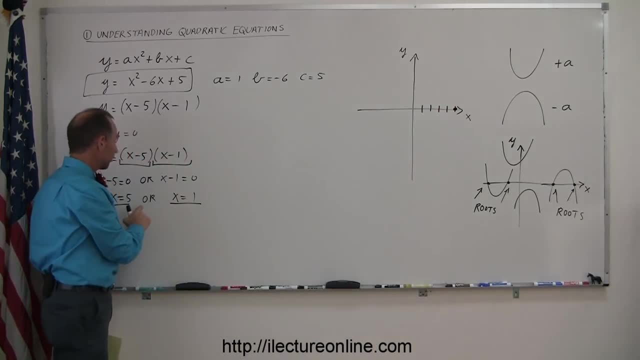 so right there, and the other place, where it crosses the x-axis, will be at x equals 1, which is right here, and those are considered the two roots of my quadratic equation. All right, now there's another thing about a quadratic equation that's very important. It's: 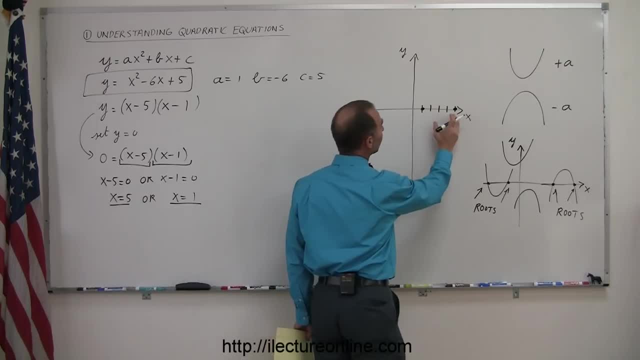 called the axis of symmetry. If I find the midway point between those two numbers, so this is 1, 2, 3,, 4, 5, and so the midway between 1 and 5 is the number 3.. If I now draw, 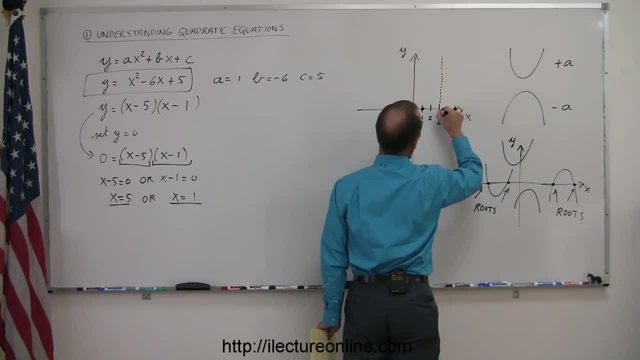 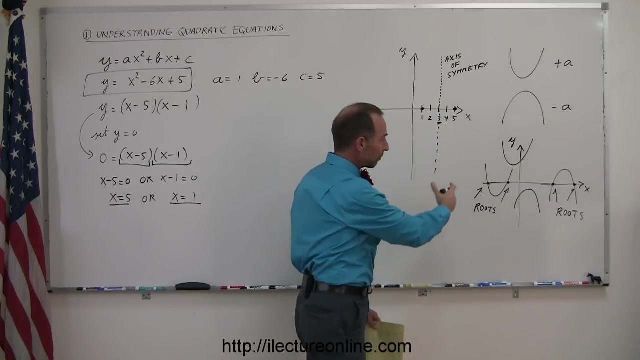 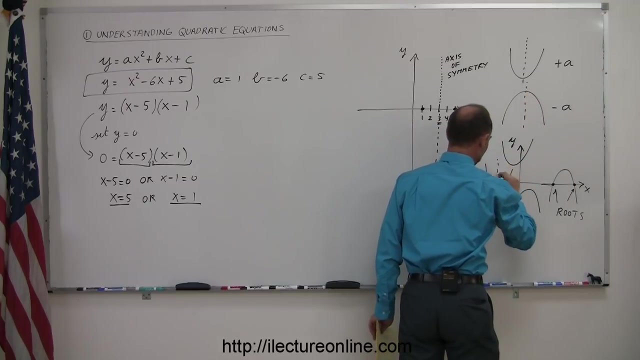 a dashed line, vertical line through the point x equals 3 on the x-axis. that is now called the axis of symmetry. And again, if you look at my examples over here, if you draw a line halfway between here and halfway between right there and right in the middle there, right in the middle there, 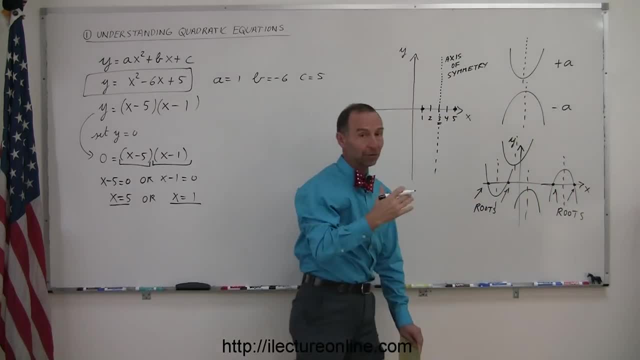 right in the middle there and right in the middle there. notice those lines are not the same. They're not the same. They're not the same, They're not the same lines. those dashed lines are the exact line that divides a parabola in two equal parts. 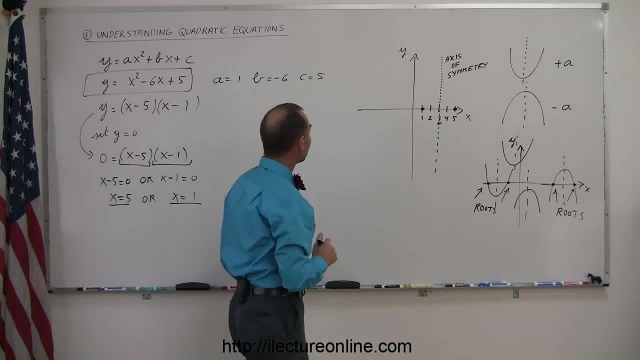 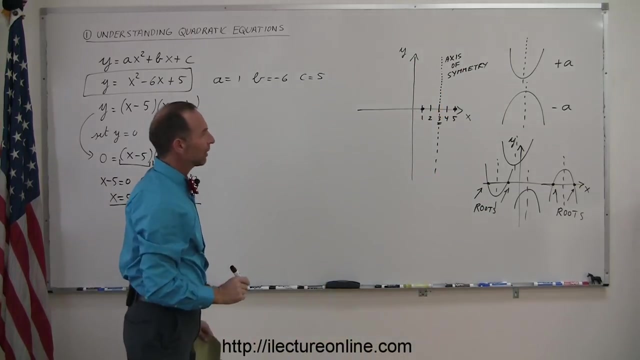 Therefore that's called the axis of symmetry. Now notice that the number from the x squared term is positive. It's a positive one. That means the parabola opens upward. That means I'm going to have a parabola that looks kind of like this: To find a few more details if I now plug in to: 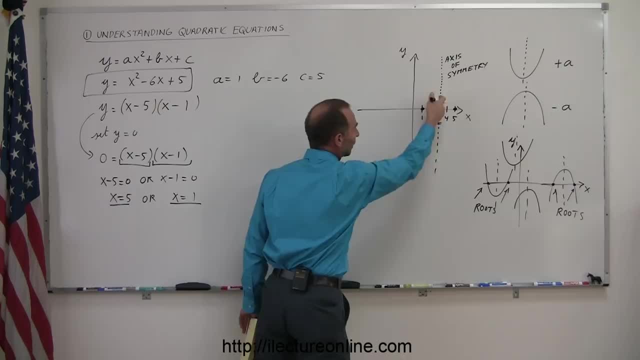 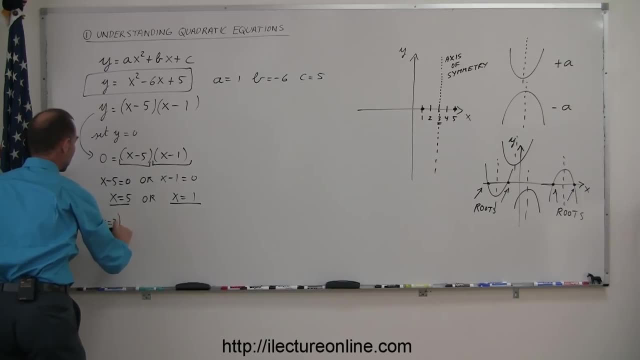 my equation, the value of x, where the axis of symmetry goes right through, in this case the number 3.. So I'm going to solve for my equation when x equals 3.. That's again the point where the axis of symmetry goes right through. Let's see what I get. So I'm taking my equation and 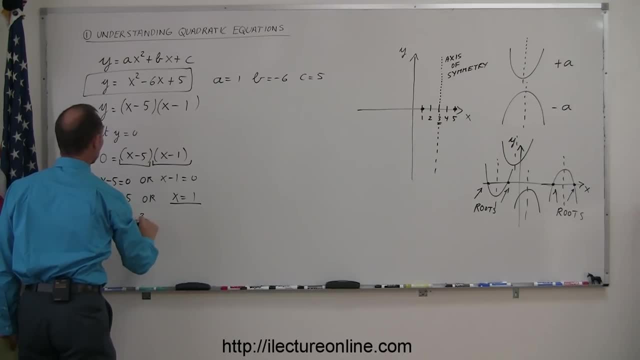 instead of x, I'm going to write a 3.. So I get a 3 squared minus 6 times 3 plus 5.. So notice, I took my original example and instead of an x, I write a 3.. Instead of this x, I write a 3.. 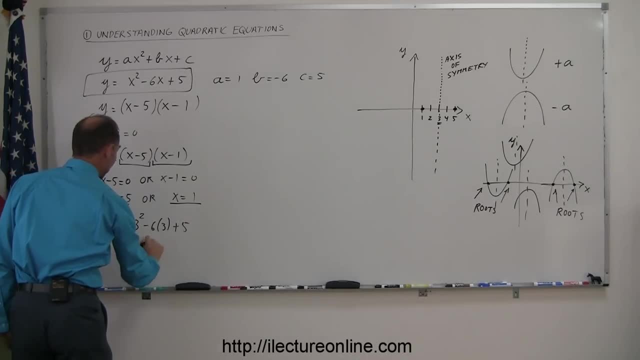 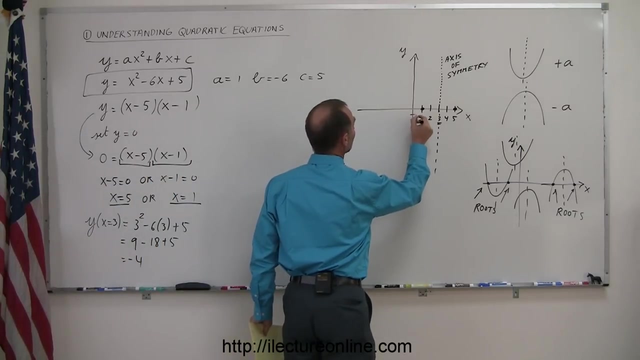 If I work that out, I get 9 minus 6 times 3 is 18 plus 5.. And so that's plus 14 minus 18.. That's equal to minus 4.. So that means when x equals 3, my y will be negative 4.. So 1, 2, 3, 4.. That's. 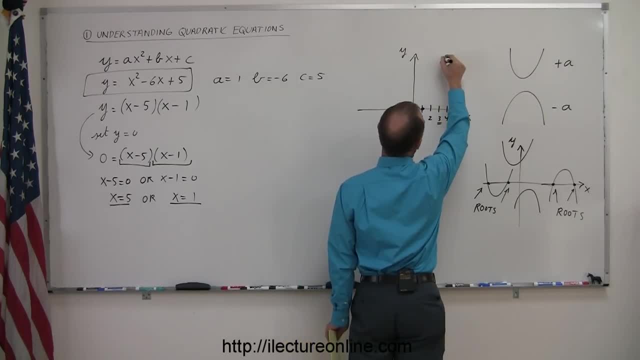 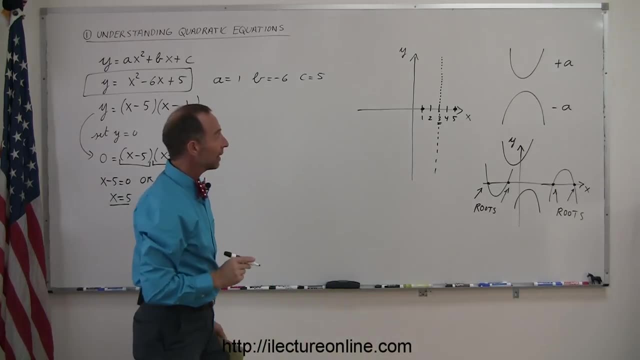 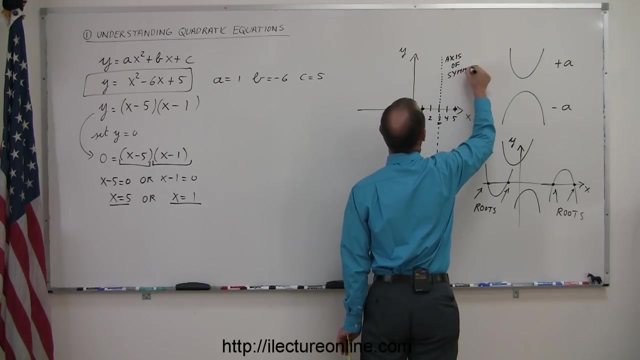 1 and 5 is the number 3, if I now draw a dashed line, vertical line through the point x equals 3 on the x-axis, that is now called the axis of symmetry. And again, if you look at my examples over here, if you draw a line halfway between: 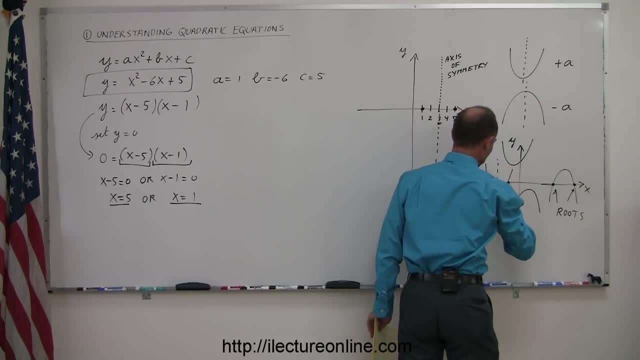 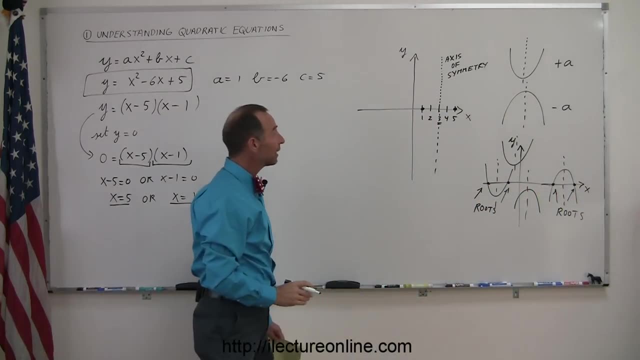 here and halfway between right there and right in the middle there, right in the middle there, right in the middle there and right in the middle there. notice those lines. those dashed lines are the exact line that divides a parabola in two. 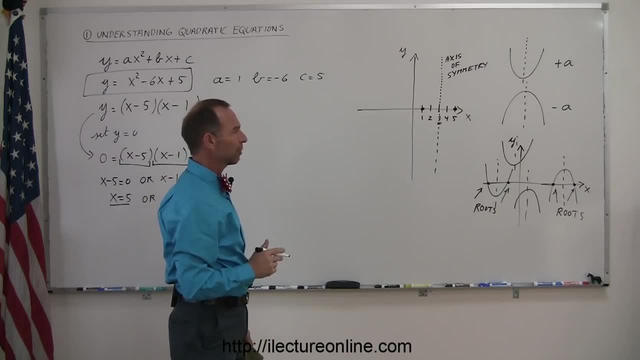 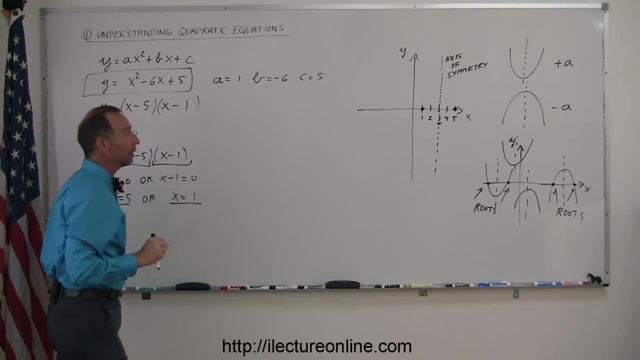 equal parts. Therefore, that's called the axis of symmetry. Now notice that the number from the x squared term is positive. it's a positive one. that means the parabola opens upward. that means I'm going to have a parabola that looks kind. 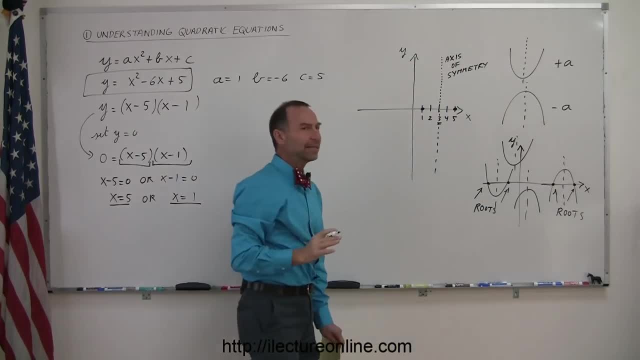 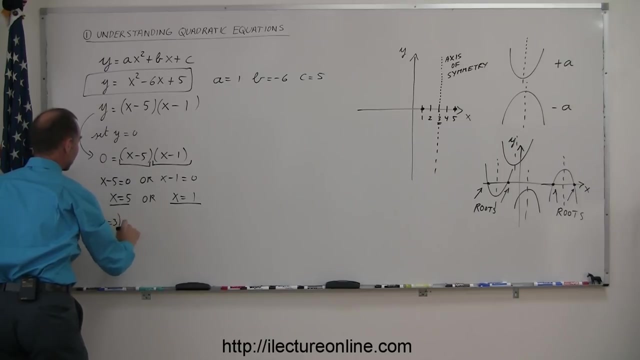 of like this To find a few more details: if I now plug in to my equation the value of x, where the axis of symmetry goes right through, in this case the number 3, so I'm going to solve for my equation when x equals 3, that's again the point where 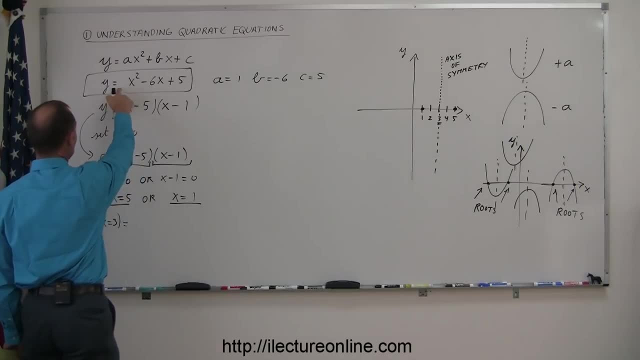 the axis of symmetry goes right through. let's see what I get. So I'm taking my equation and instead of x I'm going to write a 3, so I get a 3 squared minus 6 times 3 plus 5,. so notice, I took my original example and instead of an x I write a 3, instead of this: 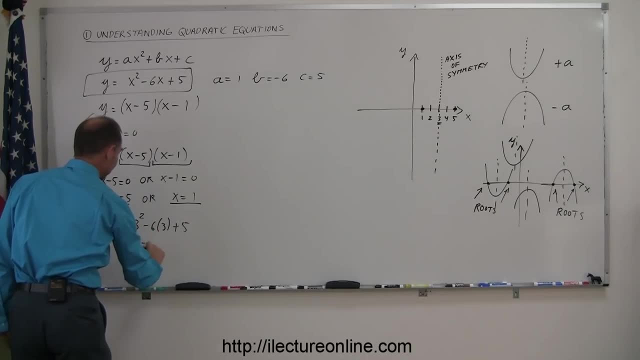 let me mark that. So I get 9 minus 6 times 3 is 18 plus5, and so that's a plus14, minus18,, that's equal to minus 4, so that means when x equals 3, my y will be. 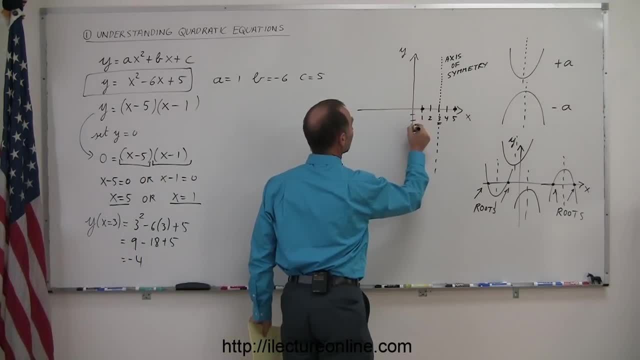 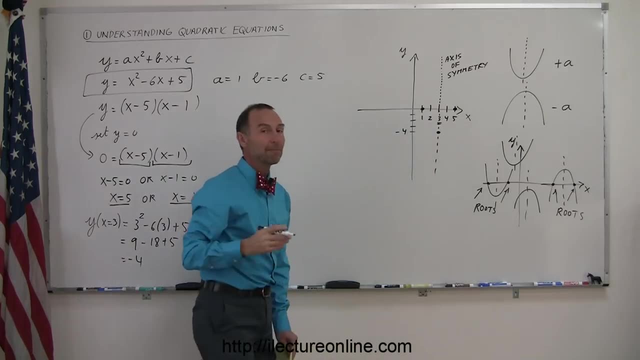 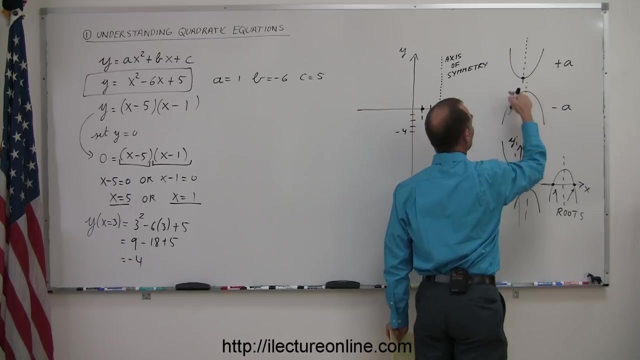 negative4, so that's negative 4 right here. so x equals 3,, y equals negative 3, that is the bottom or top point of my parabola. so if my parabola goes upward, the lowest point of my parabola is this point, right there. If my parabola opens downward, then my lowest, or in this: 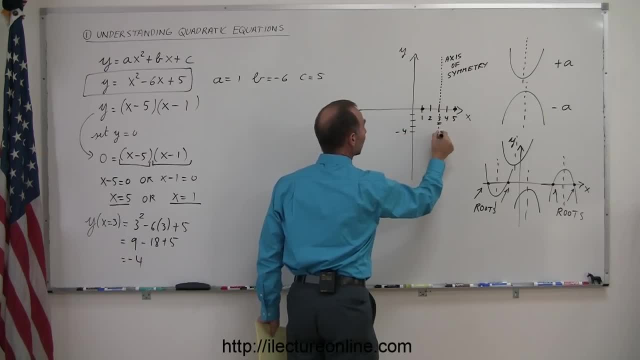 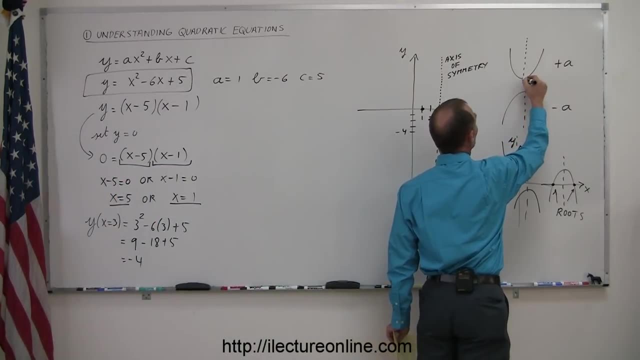 negative 4 right here. So x equals 3, y equals negative 3.. That is the bottom or top point of my parabola. So if my parabola opens upward, my lowest point of my parabola is this point, right there. If my parabola opens downward, then my 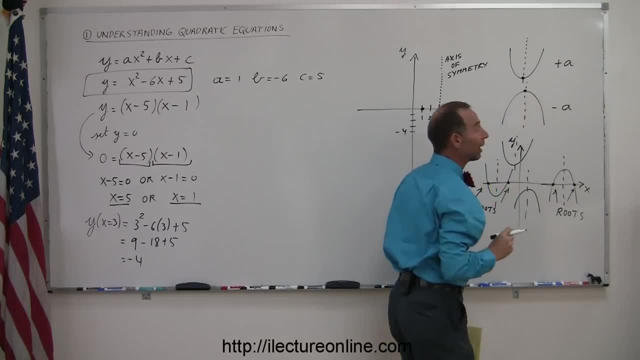 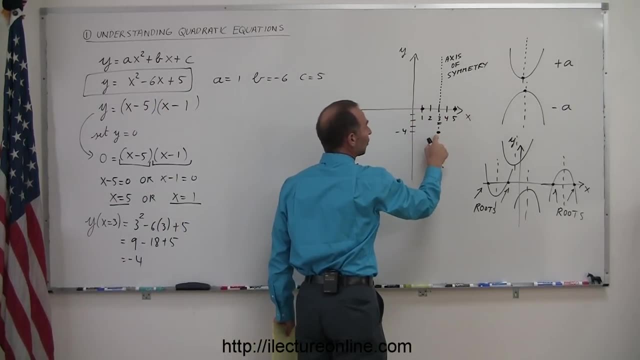 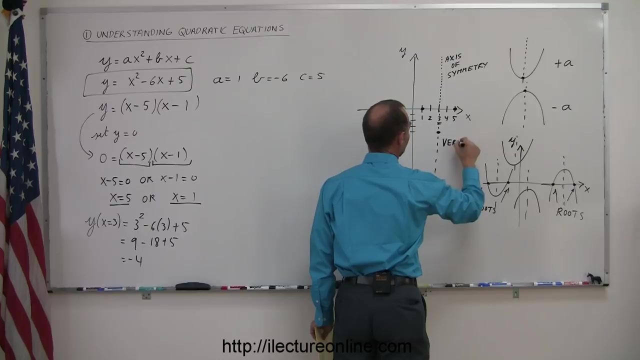 lowest, or in this case, my highest point right there, will be that point right there. So in this case, since a is a positive number, my parabola opens upward. So this will be my lowest point on my parabola, also known as the vertex. So that's the vertex of my parabola. Now there's one more. 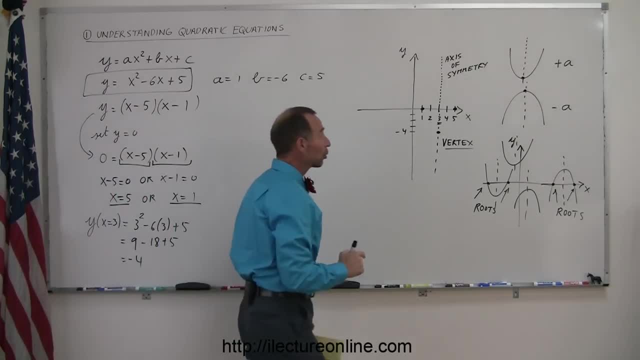 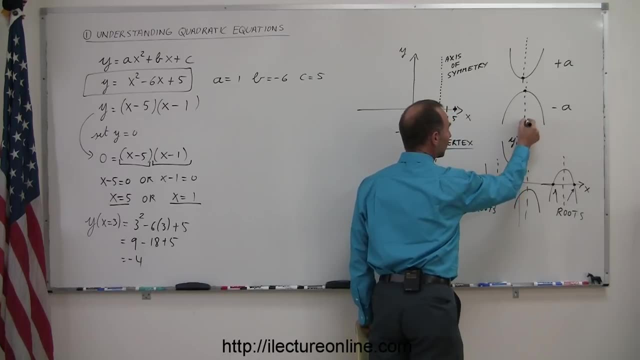 special point about the parabola. Sometimes the parabola will cross the y-axis, like over here. In this case it doesn't look like it, but if it goes on, if you keep going long enough, again, eventually you will. 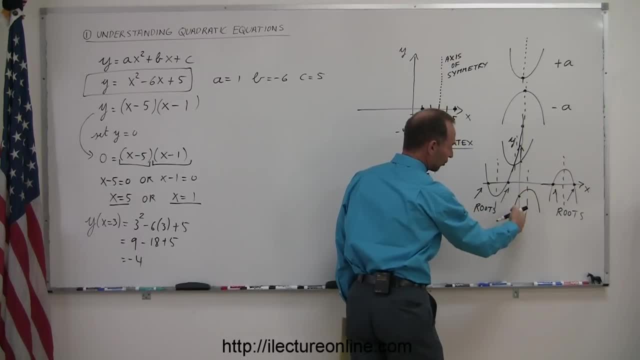 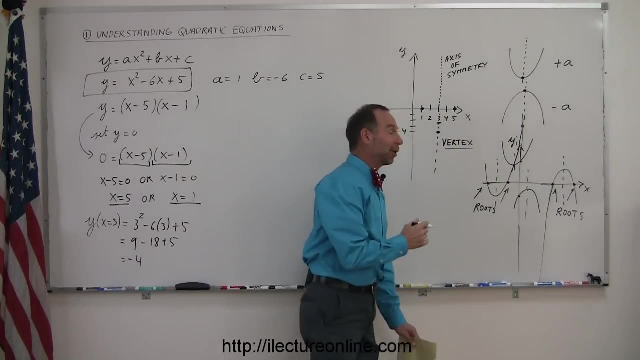 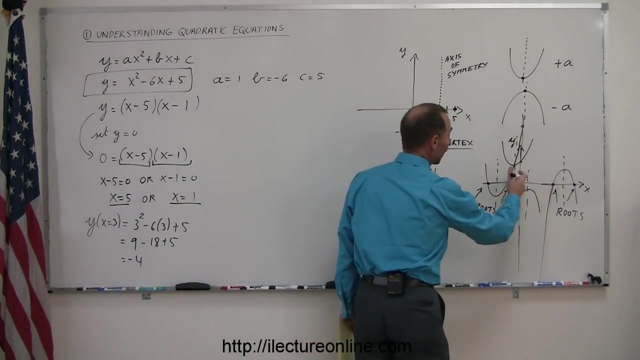 cross the y-axis Right here. this parabola crosses the y-axis over here, And if this parabola goes on long enough, eventually you can see way down here somewhere the parabola will also cross the y-axis. How do we find that point? Well, remember, any time you cross the y-axis you'll find that point. 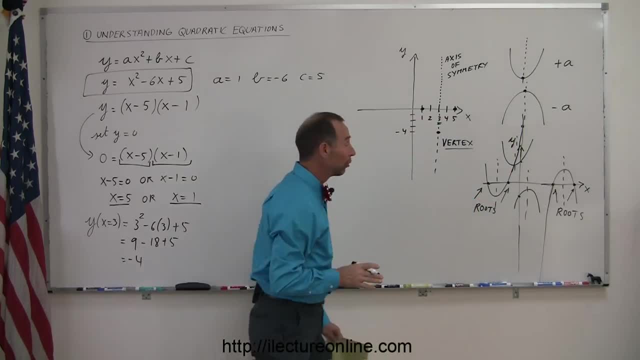 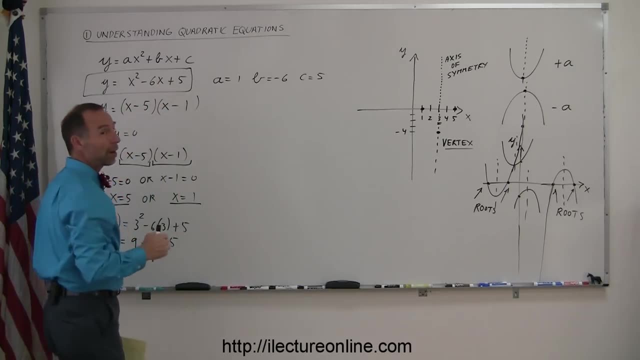 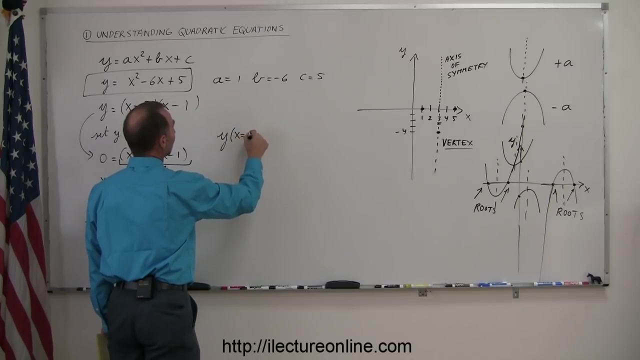 y-axis. that means that the x value must equal zero. So to find that particular point, we take our initial equation again and plug in zero for x to see where the equation or where the parabola crosses the y-axis. So I'm going to solve for y when x is equal to zero. Again I take my equation. 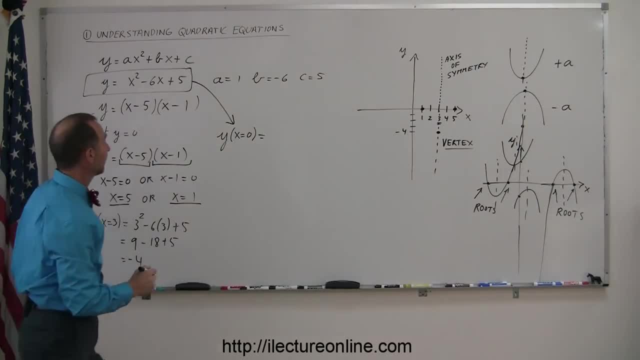 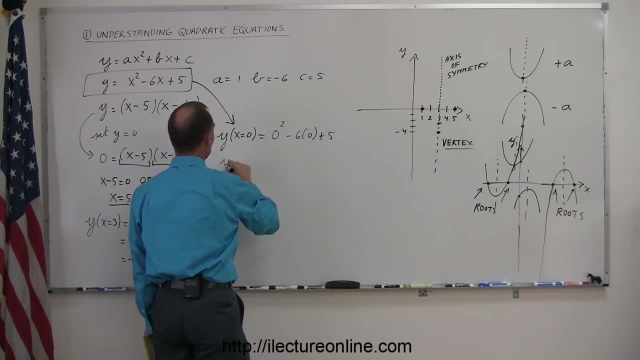 right there. plug in a zero for every x that I find. So I get zero squared minus six times zero plus five. So I get zero squared minus six times zero. I take my equation right there and plug in the zero for y: when x equals zero is equal to five. 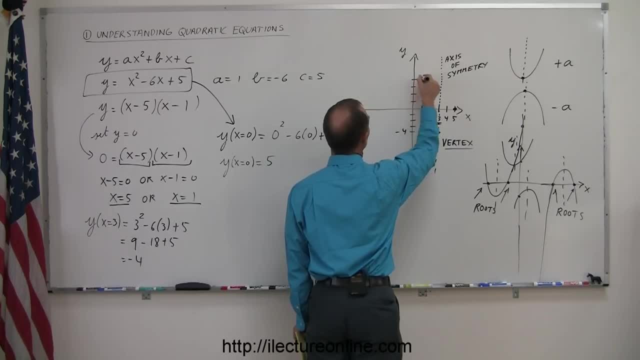 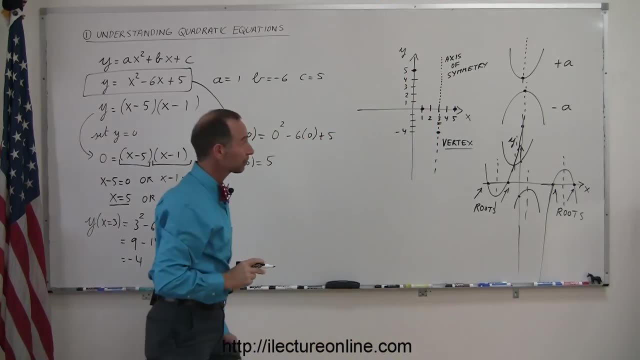 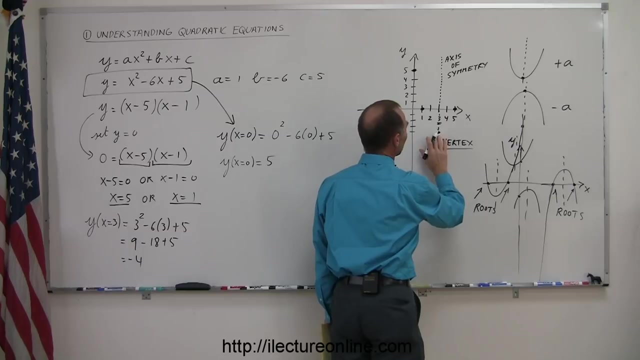 So, going to my example here, my graph: when x equals zero, my y value should be five. So it's one, two, three, four, five, And so my parabola must cross that point as well. Now notice, I have four points. I know my equation can be graphed like a parabola. Here's my lowest. 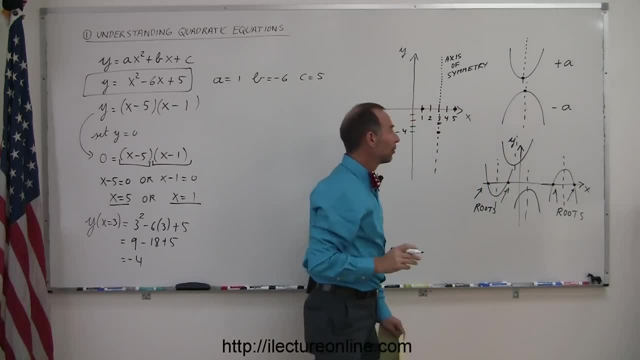 case, my highest point right there, will be that point right there. So in this case, since a is a positive number, my parabola opens upward. so this will be my lowest point on my parabola, also known as the vertex. So that's the vertex of my parabola. Now there's one more special point. 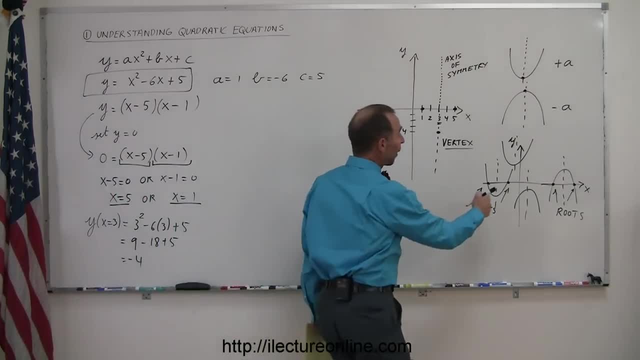 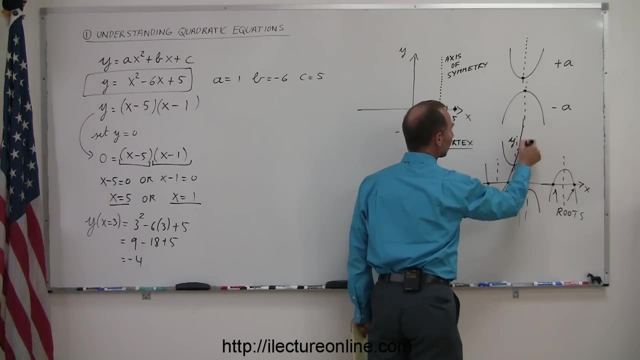 about the parabola. Sometimes the parabola will cross the y-axis, like over here. In this case it doesn't look like it, but if it goes on, if you keep going long enough again, eventually you will cross the y-axis right here. This parabola crosses the y-axis over here, and if the parabola goes on, 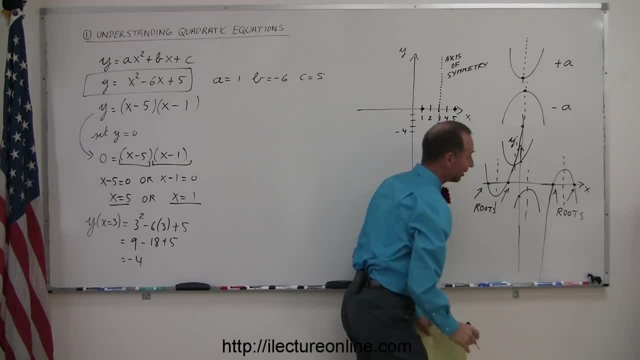 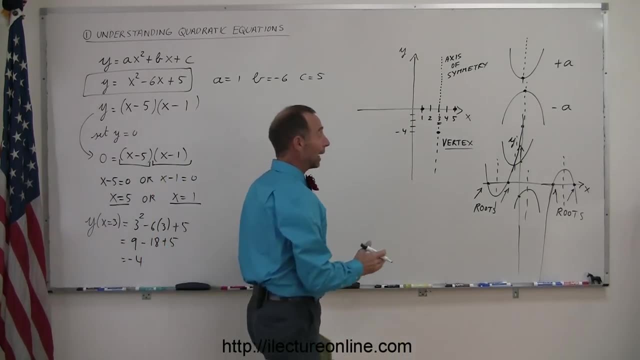 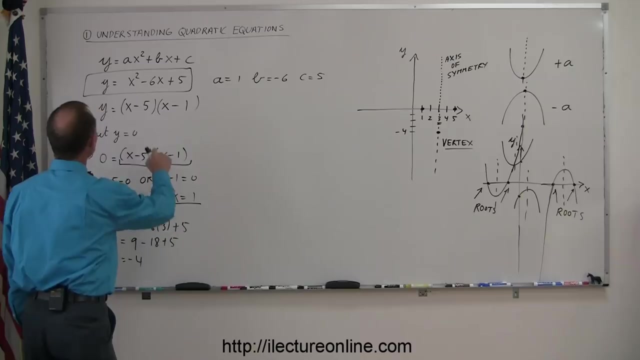 long enough. eventually you can see way down here. somewhere the parabola will also cross the y-axis. How do we find that point? Well, remember, anytime you cross the y-axis, that means that the x value must equal 0. So to find that particular point, we take our initial. 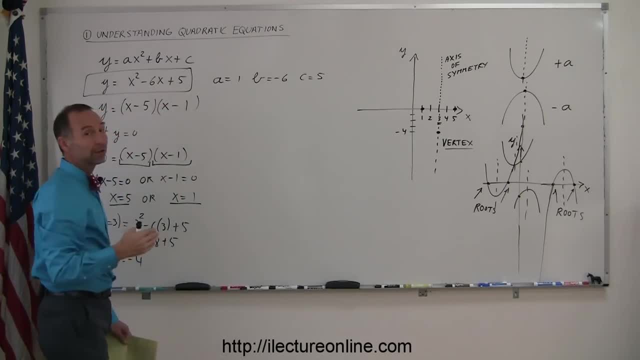 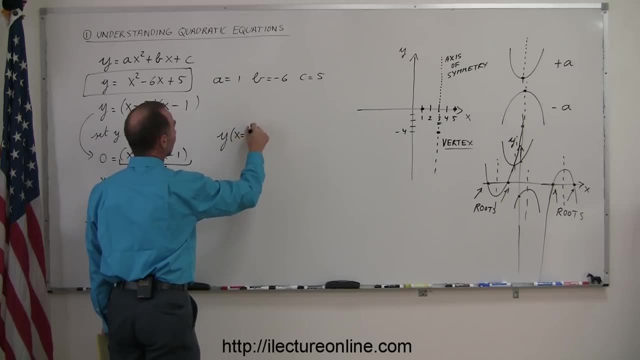 equation again and plug in 0 for x to see where the equation or where the parabola crosses the y-axis. So I'm going to solve for y when x is equal to 0. And again I take my equation right there, Plug in the 0 for every x that I find. 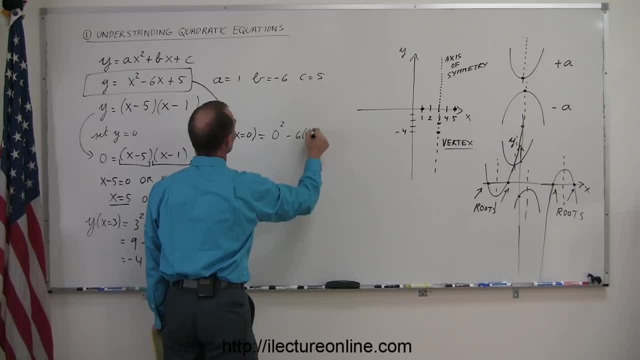 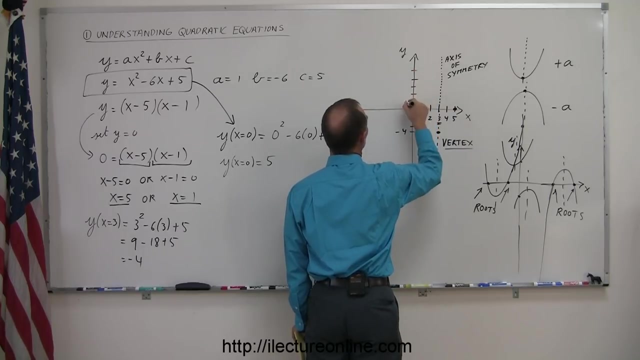 So I get 0 squared minus 6 times 0 plus 5, or y is over 5.. when x equals zero is equal to five. So, going to my example here, my graph, when x equals zero, my y value should be five. So it's one, two, three, four, five, and so my parabola must cross. 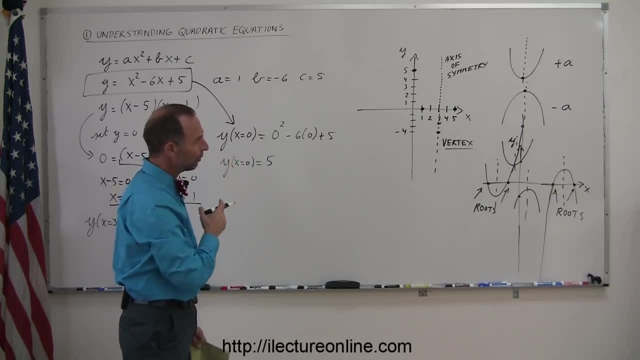 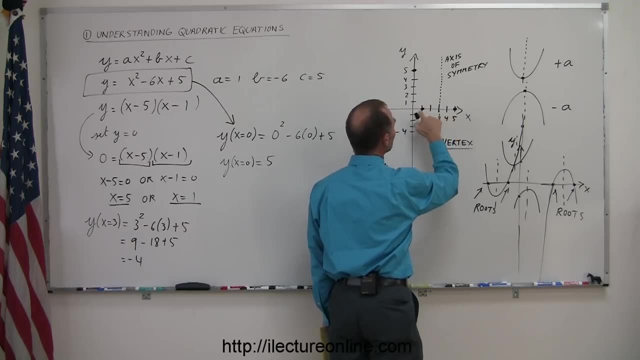 that point as well. Now notice, I have four points. I know my equation can be graphed like a parabola. Here's my lowest point, or the vertex. There's my two roots, There's the point where the parabola crosses the y-axis. If I now carefully connect all those dots with a free hand like that, 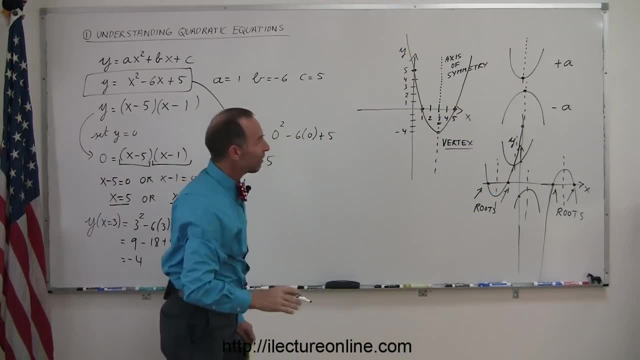 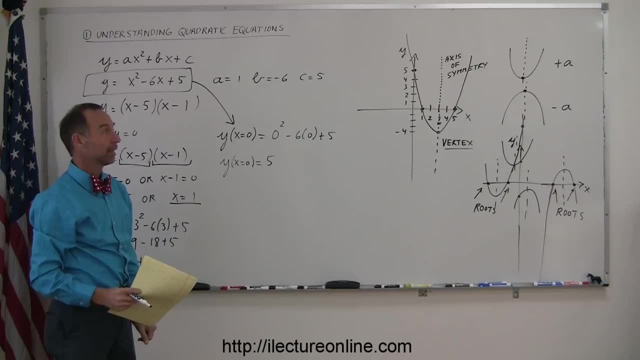 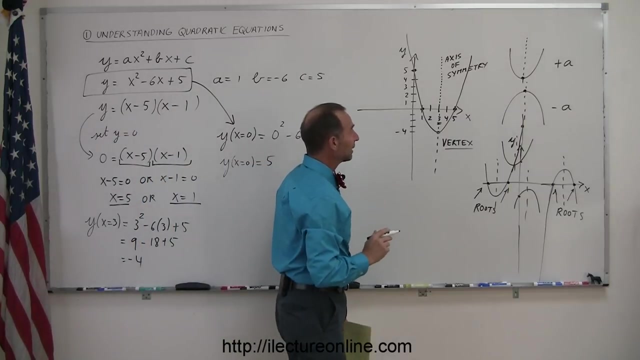 I have now drawn a graphical representation of my example right here, my quadratic equation, and you can see how that looks like a nice parabola. So that's what a parabola is, That's what a quadratic equation represents, And if you want to look at the points very carefully again,